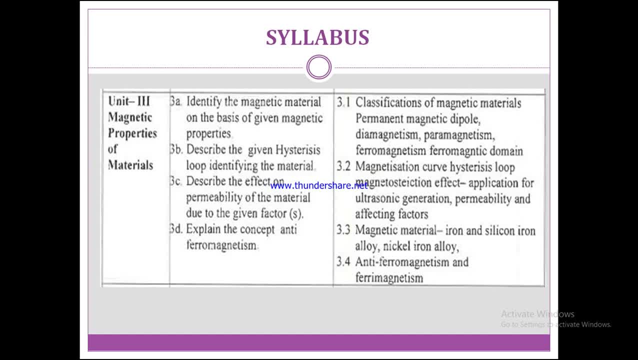 student should be able to identify the magnetic materials on the basis of given magnetic properties. Next unit outcome is: describe the given hysteresis loop identifying the material. Unit outcome number three, that is, 3C, describe the effect on permeability of the material due to the 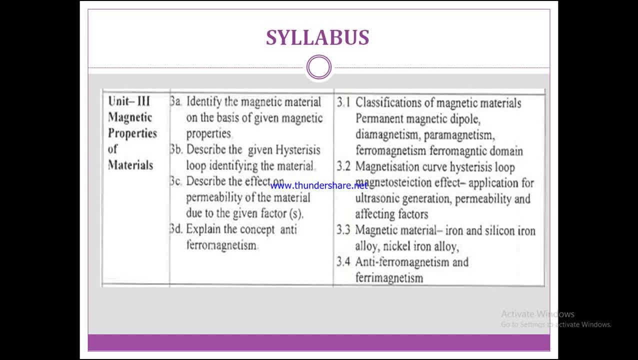 given factors And unit outcome. number four, that is 3C, describe the effect on permeability of the material. That is 3D: explain the concept of anti ferromagnetic. Now this unit is distributed in five main topics, such as topic number one, that is nothing but classification of magnetic. 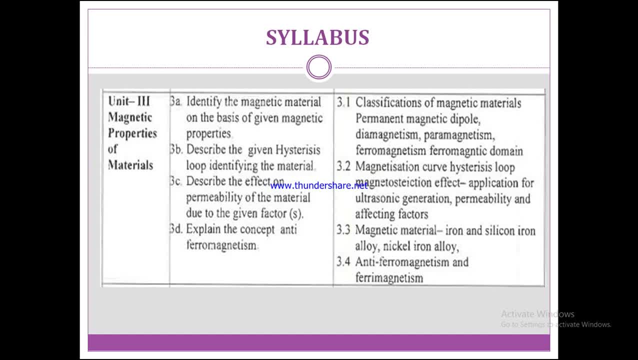 materials, Permanent magnetic dipole, permanent magnetic dipole and permanent magnetic dipole, Dimagnetism concept, paramagnetism concept, ferromagnetism concept and ferromagnetic domain. Next topic is magnetization curve, hysteresis loop- magnetostriction effect: application. 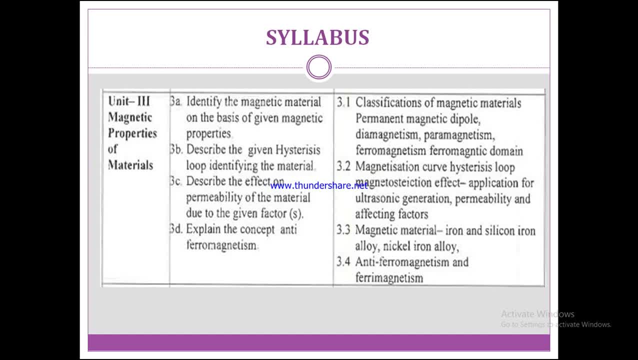 for the ultrasonic generation: permeability and affecting factor. Next topic is nothing but magnetic materials: iron and the silicon iron alloy, nickel iron alloy. The last topic is nothing but anti ferromagnetism and ferromagnetism concept. Now let's start to discuss. 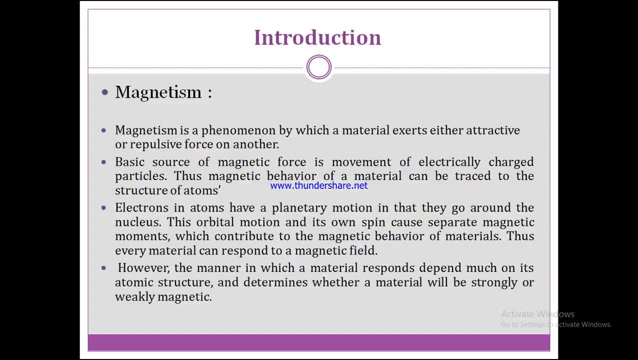 Unit number three with the basic concept. Now, in the introductionary part, we are going to discuss the concept of magnetism. Magnetism is a phenomenon by which a material exerts either attractive or a repulsive force on another. Basic source of magnetic force is movement of electrically charged particles. Thus the 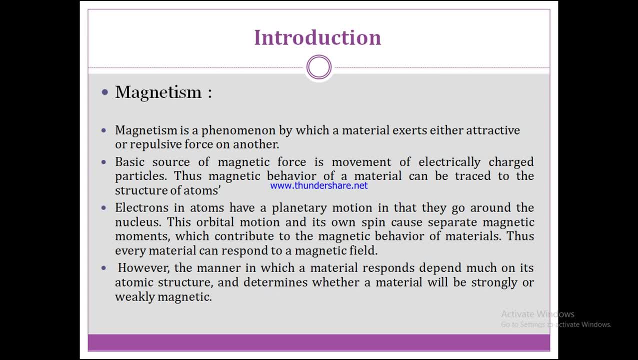 magnetic behavior of a material can be traced to the structure of atom. Electrons in atoms have a planetary motion in that they go around the nucleus. This orbital motion and its own spin cause separate magnetic moments which contribute to the magnetic behavior of materials. Thus every material can respond to a magnetic field. 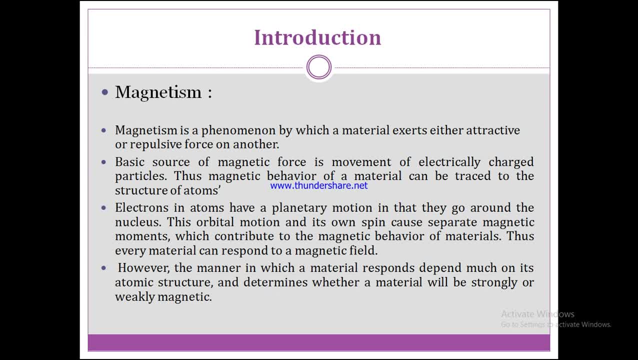 However, the manner in which a material can respond to a magnetic field is not the same. A material response depends on much on its atomic structure and determines whether a material will be strongly or weakly magnetic. Now we can start the definition of the magnetic materials. 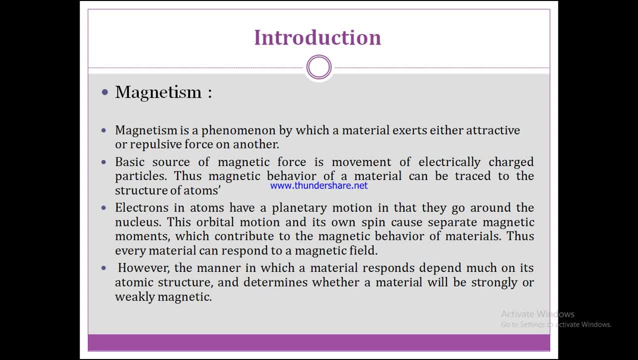 Now the materials in which a state of magnetism can be induced is called as magnetic materials. Now the magnetism is a phenomenon by which the material exerts two types of forces. in that material, Either the force is having the attractive type or it should be having the repulsive force type. 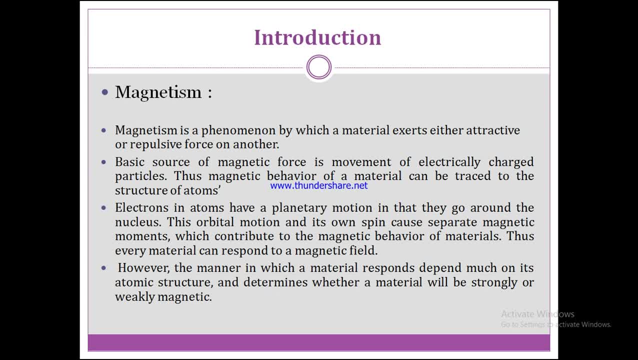 The main concept behind this magnetism is that the magnetic force movement is an electrically charged particles. which behavior of that material should be dependent? It depends upon the structure of an atom. Now, the electrons in an atom have a planetary motion in the orbit that they go around the nucleus. 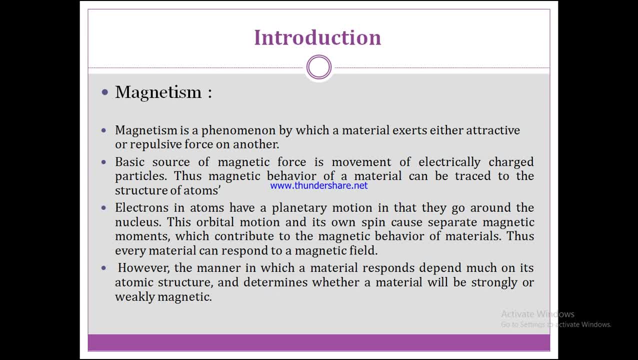 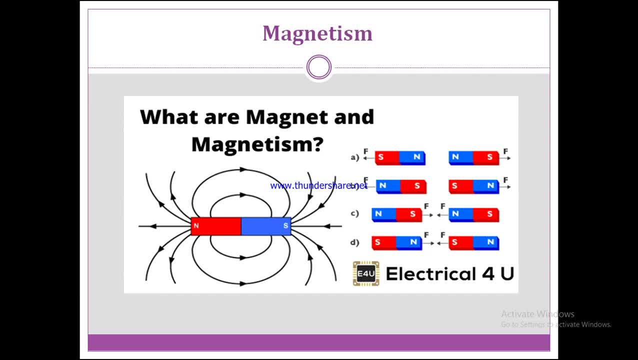 Also, it have its own spin around itself. causes to a separate magnetic moments, which contributes to the magnetic behavior of material. Also, it have its own spin around itself. causes to a separate magnetic moments, which contributes to the magnetic behavior of material. the poles which are placed near to the each other according to our application. 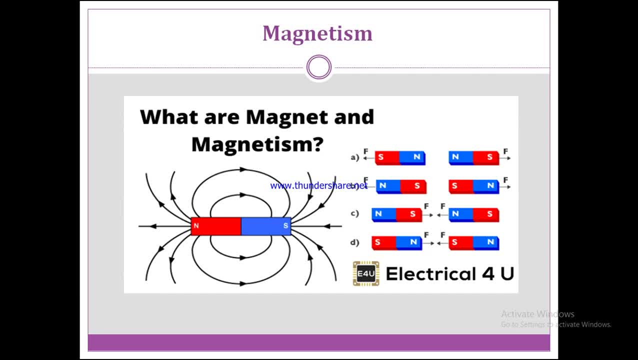 now if we can connect or we can place the two same poles in between. a smaller distance between them then, and a repulsion force is to be introduced by that magnet. and it is indicated that in first diagram of this slide that should be nothing but figure number a, when a magnet having the poles of s and n, 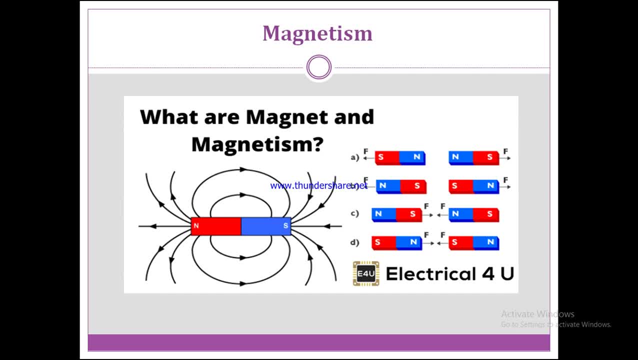 and another magnet having the poles of n and s are kept together, then two similar poles are available near to the each other. now, in this situation, the repulsive type of force is introduced among these two magnets and hence force exerted on that magnet is having opposite force direction due to that magnitude. now it not only happens. 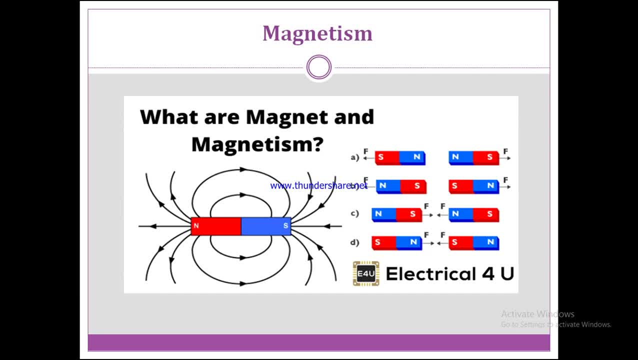 with North Pole only, but also with other magnet has opposite magnet direction and then we can insert the two magnets as it is shown in the slide only, but it also happens with the S pole and that situation is indicated with B diagram. When N and S magnet, it should be kept near to S and N magnet, then also two similar poles. 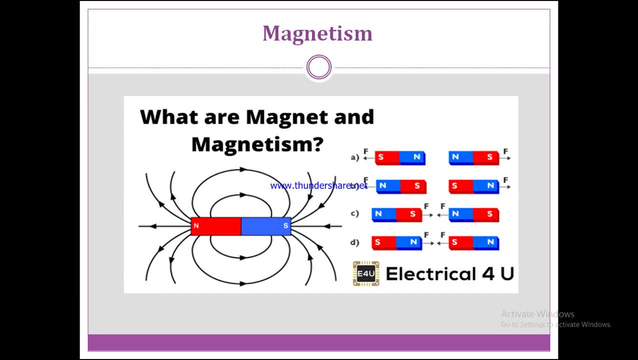 that is nothing but S in this situation is kept together and because of that the same polarity of magnet- it should be- introduces the repulsion type of force between these two and hence over here the force exerted on two magnets is having the dependent force in different directions. due to that, the repulsion type of force is introduced when A and B situation. 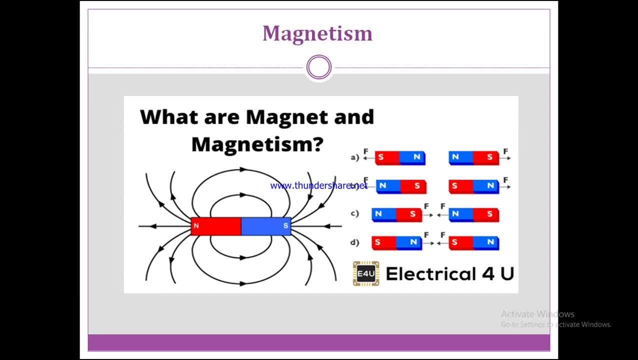 will be there. Now in the third diagram, that is, N and S, it should be kept to another N and S pole of the magnet, then S pole and N pole. These are different with each other, the different poles of each other. and now, according to the 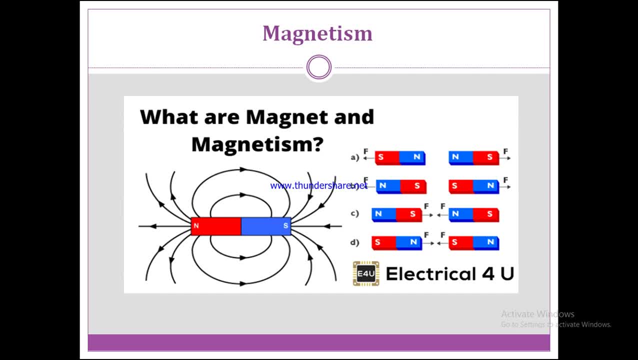 magnetism concept. the different poles should be creates the attractive type of force between the magnets and it should be indicated with the attraction type of force which are getting closer to that force. The force should be indicated with diagram number C and when fourth combination should be there, that should be nothing but S and N pole of a magnet. it should be having the 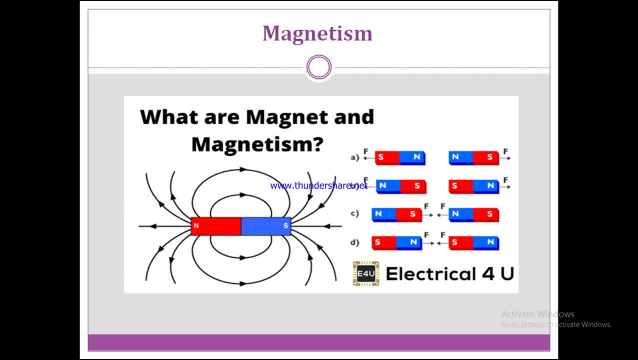 another magnet that is nothing but S and N, Then the N pole is near to the attraction type of force. If the attraction type of force is nearly closing to the S pole and because of two opposite poles are kept together, then the attraction type of force is to be created between these. 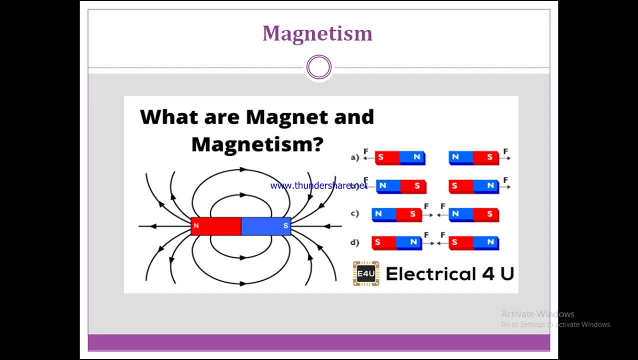 two magnets and hence the force produced by that two magnet, it should be attracted towards each other. Now from this diagram we can take an conclusion that when, When, When The two magnets having the same poles near to each other should be creates an repulsion. 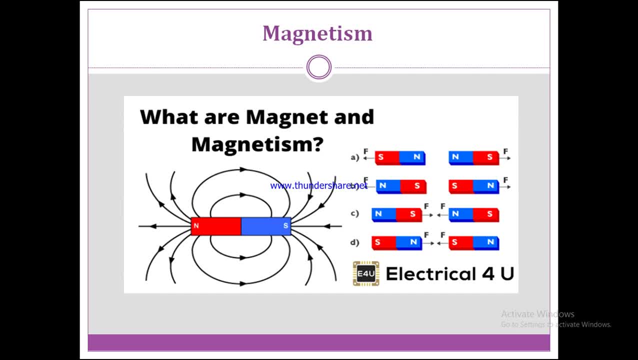 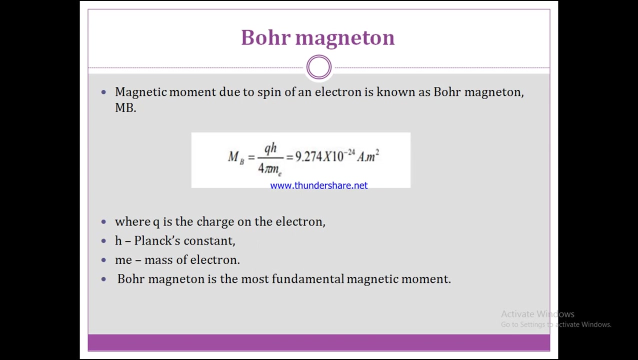 type of a force. and when two magnets having different type of poles closing to the each other, then that magnet should be creates an attraction type of force. 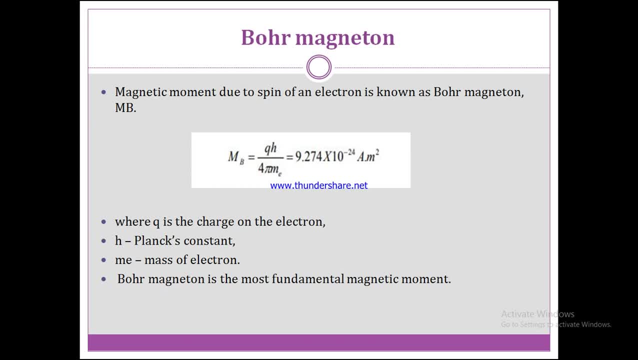 The magnetic moment due to the spin of an electron is known as Bohr's magneton. It is indicated by capital MB. We have an equation of MB that is: MB is equal to Q into H divided by 4 Pi ME. again, we have to be revise this one. mb is equal to q into h divided by 4 pi m e. 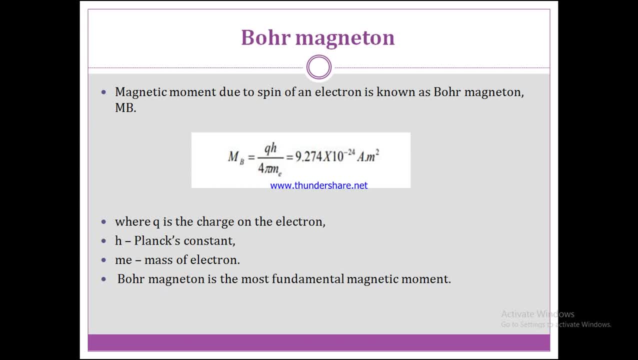 when we can put all the values regarding with this equation we can get the actual value of Bose. magneton is equal to 9.274 into 10 raise to minus 24 ampere meter square now in this equation, that is nothing but mb is equal to q into h divided by 4. pi, m, e. in this equation: 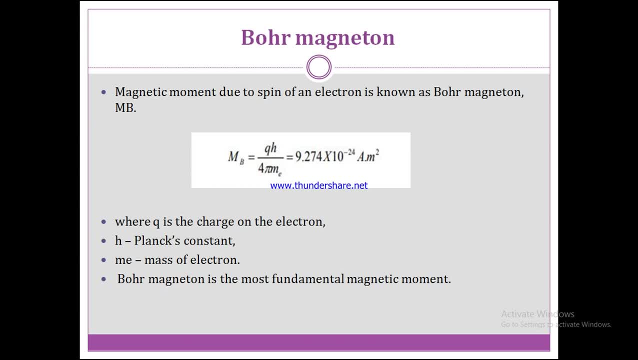 small q is small q is the charge which are present on that electron. small h is nothing but the Planck's constant. m, e is nothing but mass of an electron and according to that we have an, a value of 9.274 into 10. raise to minus 24 ampere meter square now the Bose magneton. 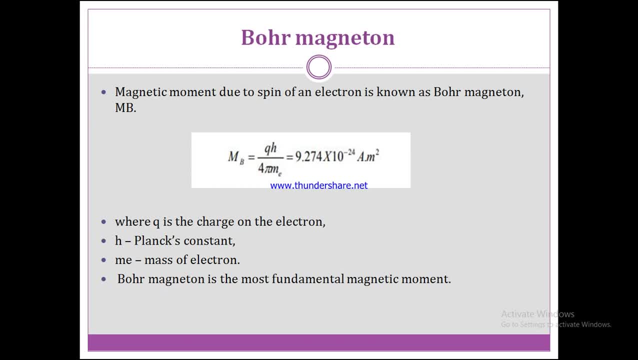 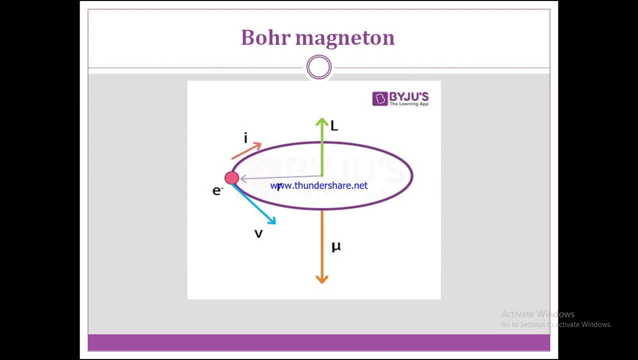 is the most fundamental magneton in the entire system as per the magnetic material is to be concern when gradually increasing of given wys� rolax. Bose magneton is the most fundamental magnetic movement. bose magneton we have discussed in deep siska rewind magnetic movement. 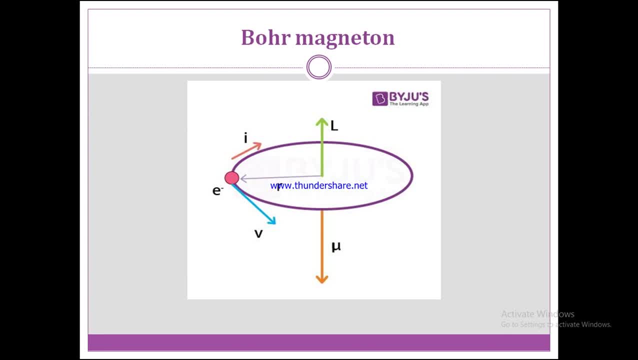 in this diagram. Now, in this diagram we have the nucleus present at the center of this circle where the length l arrow should be introduced. The initial position of that nucleus should be present at the center of the circle, having particular distance of radius r of an electron which should 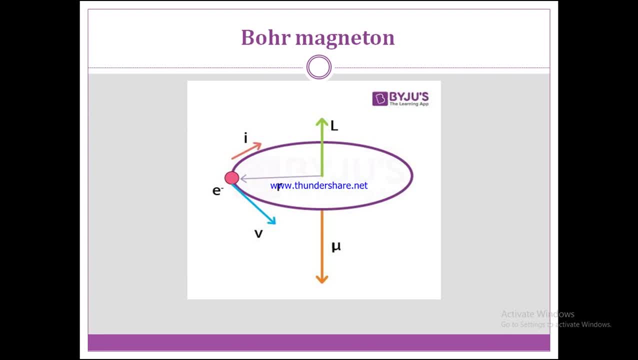 be present to the orbit. The electron is having negative charge, which are continuously moving around the nucleus. with an orbit, The electrons are moving according to the stationary velocity of the nucleus Indicated by small v, and when the electron is break down its orbit and moving towards. 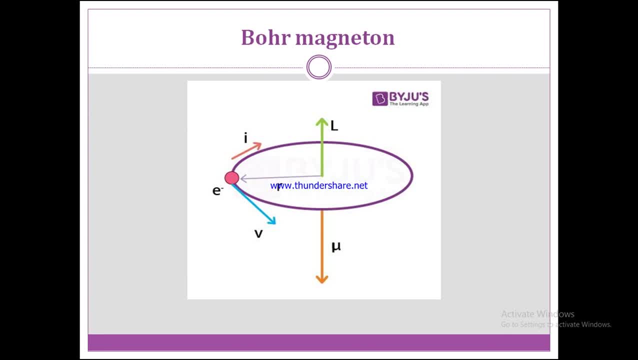 an another. electrons for the conduction of flow should be indicated by small i. that is nothing but the current which are introduced by electron. Now, the mu is nothing but the parameter. The definition of the permeability is that permeability is defined as the ability of 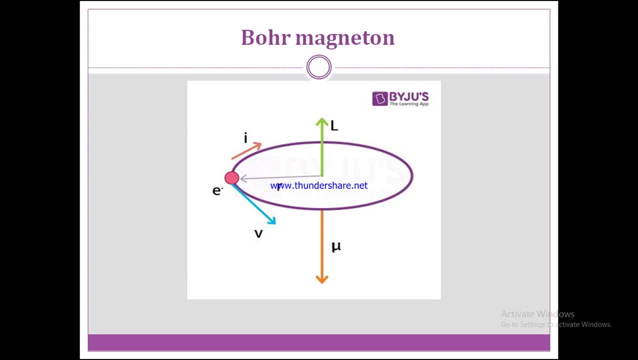 a material to easily allow the magnetic lines to pass through it. Permeability is defined as the ability of a material to easily allow the magnetic lines to pass through it. Now, the magnetic materials have high permeability, whereas the non-magnetic materials have low. 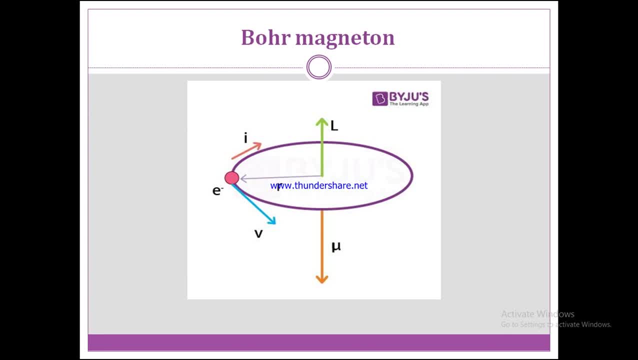 permeability, which are denoted by mu. Now over here the mu is directed towards an downward direction, whereas L it should be indicated in upward direction. Now the Bose magneton should be introduced as that when an electron is moving around the nucleus in a particular way, ie in an orbital motion, then the electron also spins. 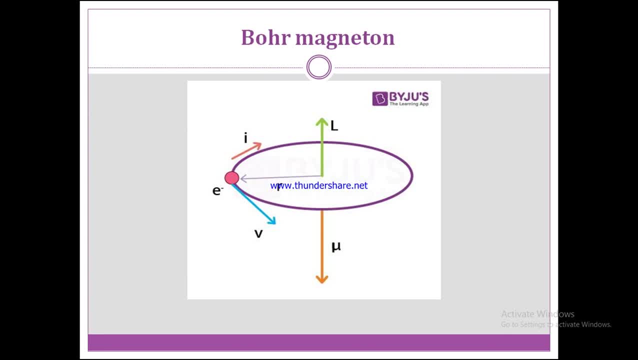 around itself, having some velocity With And a particular direction Now, according to the orbital motion around the nucleus and the spin around itself, should be creates an magnetic movement which should be cohesives to the magnetism property. It should be introduced by Bose magneton. 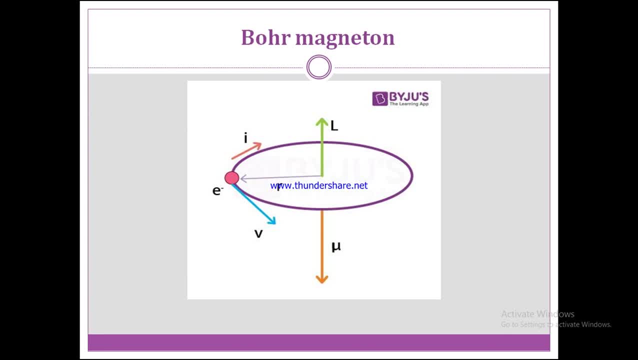 Okay, So this is how The magnetism concept has been introduced. Again, we have to be discussed the same concept for the better understanding. when an electron is having the spin around itself in anticomposite direction, then the permeability it should be created by the magnetism property. 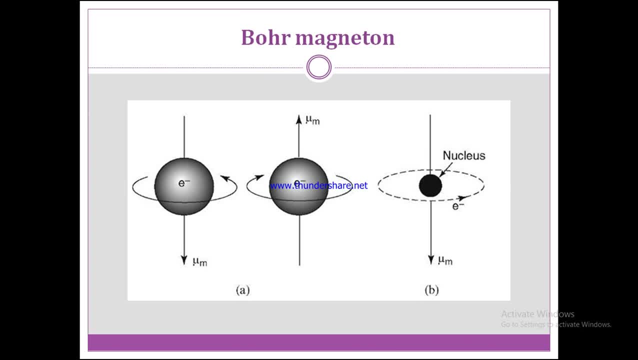 It should be created and downward direction itself. And when The electron speed in choose direction then the permeability of that magnetic material be indicated by new m is having and four direction. The electrons present in that orbit moving around the nucleus as well as the electrons are seeing 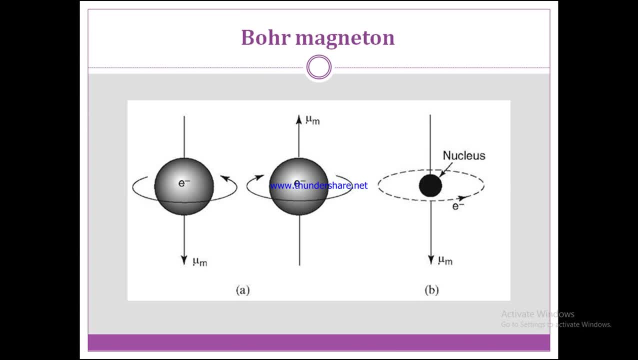 around itself and according to that, the magnetism, magnetic moment, is to be present in that material. now in the figure number b, the nucleus should be indicated with a black spot, black circular spot. the dotted line is nothing but the path where electrons are moving around the nucleus. 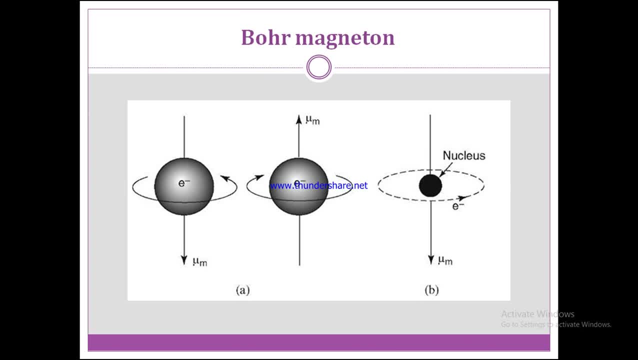 and according to that in antemnopause direction and the permeability produced by that magnetic material should be introduced or indicated in the downward direction. now, according to the bose magneton concept, the electrons which are moving around the nucleus is having the proper of pin of electron around itself in ascending with the nucleus should be. 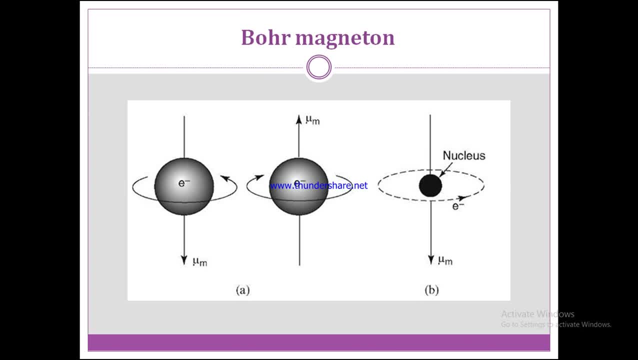 creates an magnetic moment and the net magnetic moment will be introduced by magnetic material with the help of magnetism. the number of flux lines would be created by magnetic moment is depends upon the electron spin magnetic moment and the nucleus which are attached to that electron will be. 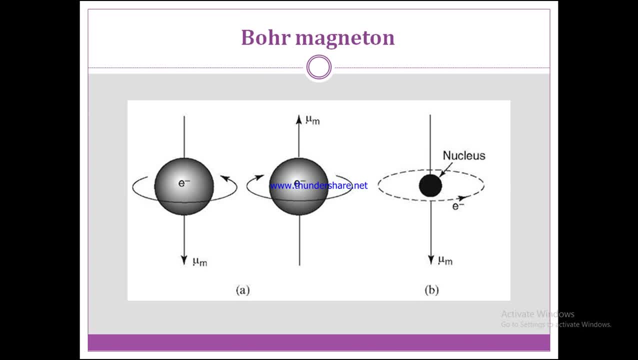 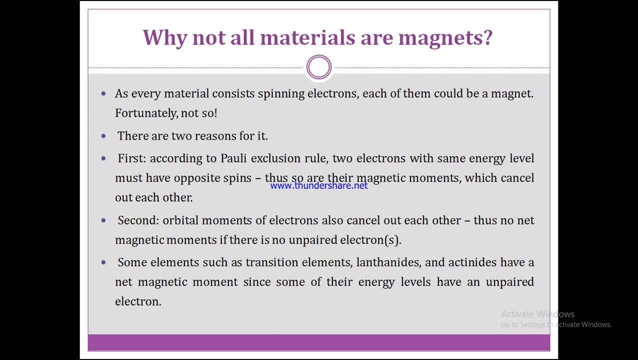 present in that atom. now the question is that, why not all materials are magnet? now the question is that, why not all materials are magnet? now the question is that, why not all materials are magnet? if the Bose magnet magnet on concept is available in each material is magnetic. 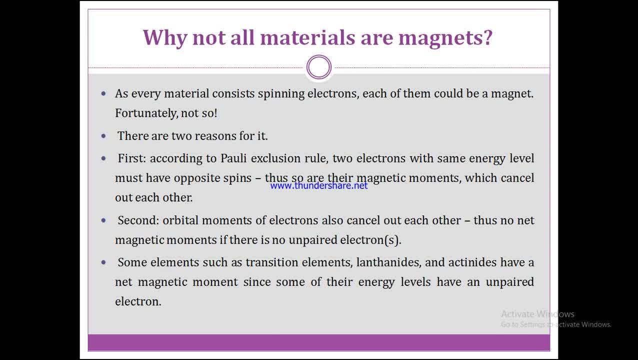 if the Bose magnet, magnet on concept, is available in each material, is magnetic material, then why not? all materials are magnets? okay, as every material consists the spinning of electrons. each of them wouldn't could be a magnet, fortunately. but this is not so. but this is not so. 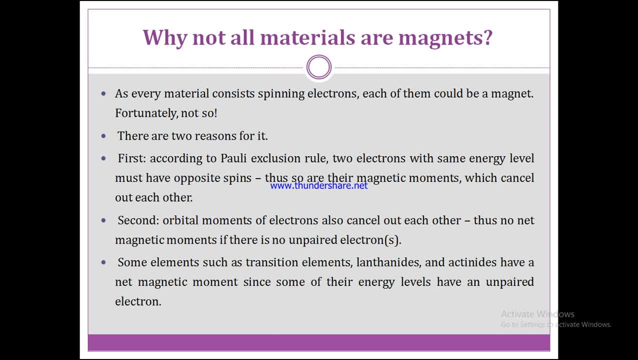 because there are two main reasons for it. the first one is, according to the poorly exclusion rule to electrons with the same energy level must have the opposite spin with each other. thus so are their magnetic moments, which are cancel out each other. means what? according to the Pauli exclusion rule, when two electrons having 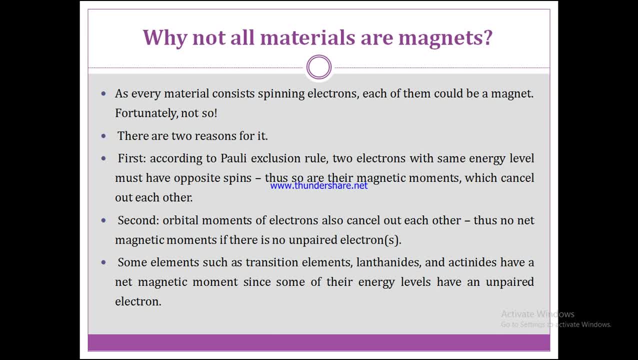 the same energy band with the opposite spin with each other, then the magnetic moment created by that electron is having the value of zero, or the force which are generated in opposite directions. they will be cancelled with each other and the net resultant becomes zero. the second reason is: 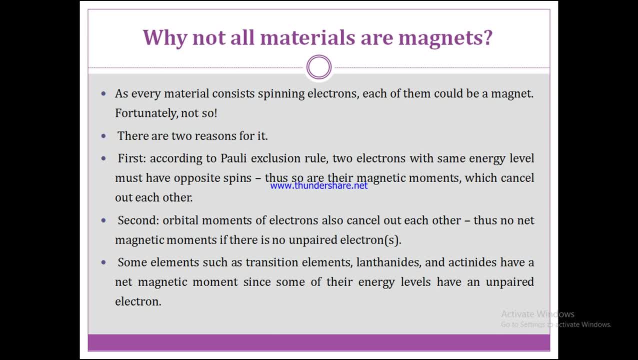 that orbital moments of electrons also cancel with each other, thus no net magnetic moments. so net magnetic moments, if there is no unpaired electrons, becomes zero. the second reason is that the orbital moments of electrons also cancel out each other and hence the net magnetic moment becomes zero. and that's why the 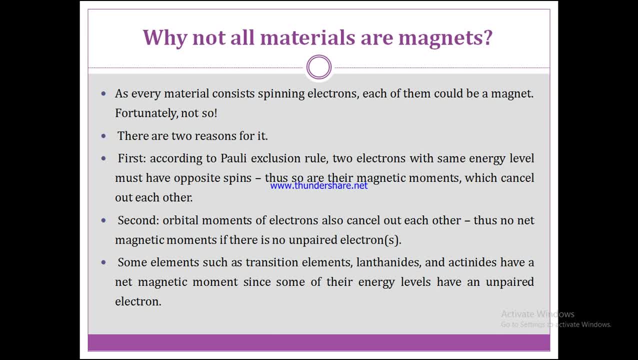 material cannot be identified as in a magnet. now, the some elements, such as the transition elements, such as the transition elements such as the lengtheners and actinides, have the net magnetic moments, since some of their energy levels have an unfair electron elements, such as transition elements that lengtheners and actinides have. 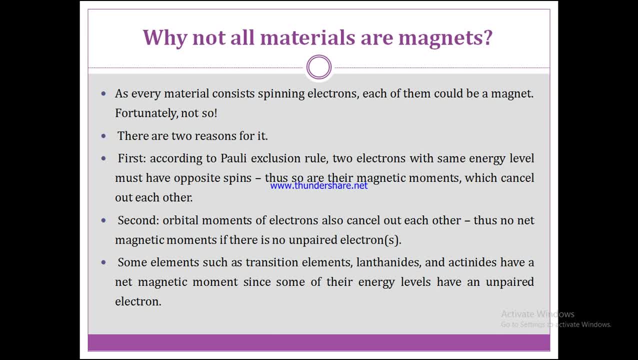 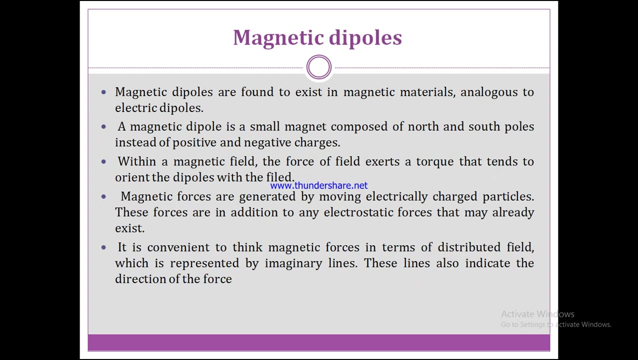 the net magnetic moments. It means some of their energy levels have an unpaired electron, Now magnetic dipoles. The magnetic dipoles are found to exist in magnetic materials analogous to electric dipoles. A magnetic dipole is a small magnet composed of north and south poles. instead of positive and negative changes, 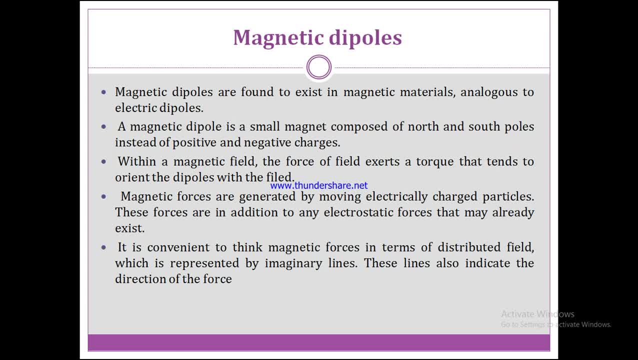 When, within a magnetic field, the force of the field exerts a torque that tends to orient the dipoles with the field. Magnetic forces are generated by moving electrically Charged particles. these forces are in addition to any electrostatic forces that may be already exist. 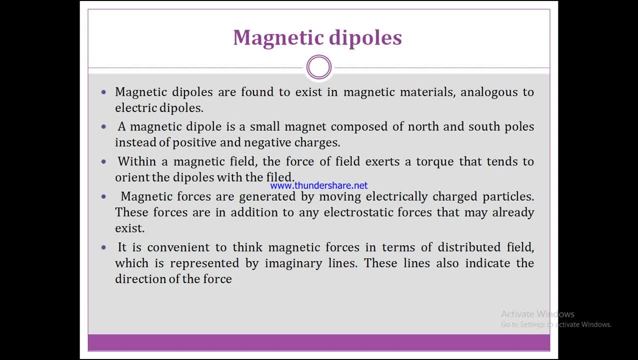 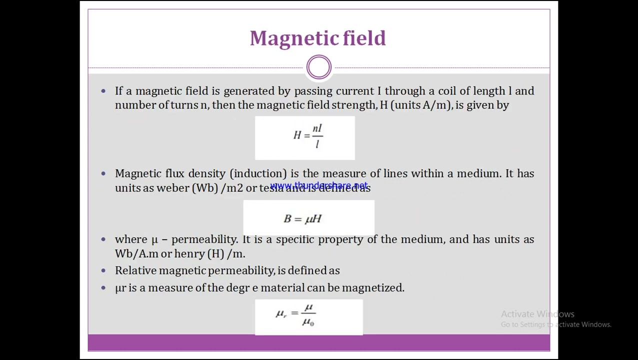 It is convenient to think magnetic forces in terms of destructed field, which is represented by imaginary lines. These lines also indicate the direction of the force. Okay, So we have an equation of. Okay, So we have an equation of. 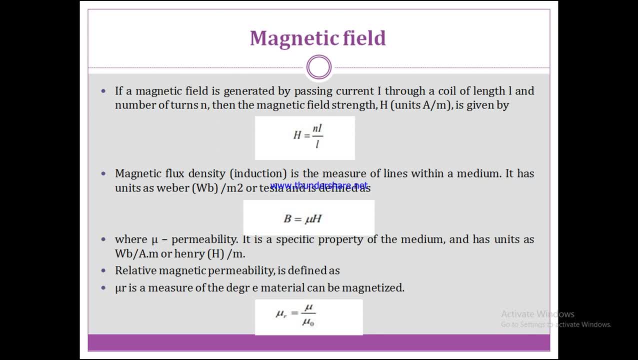 various parameters. If a magnetic field is generated by passing current I through a coil length of L and the number of terms that is nothing but N, then the magnetic field strength H should be indicated by capital H. Then the magnetic field strength H should be indicated by capital H. 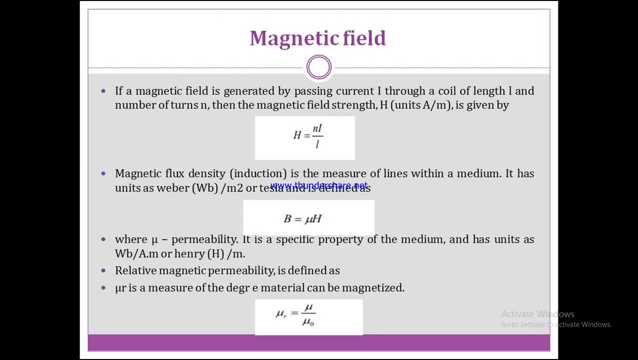 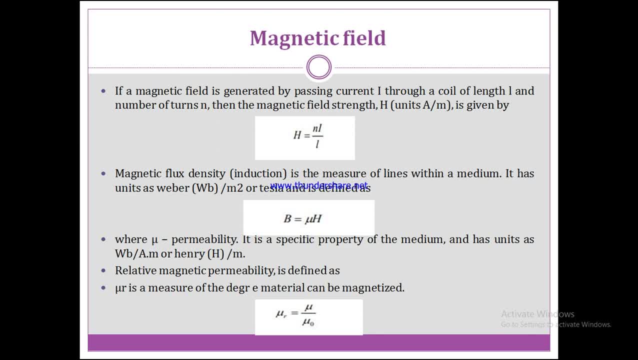 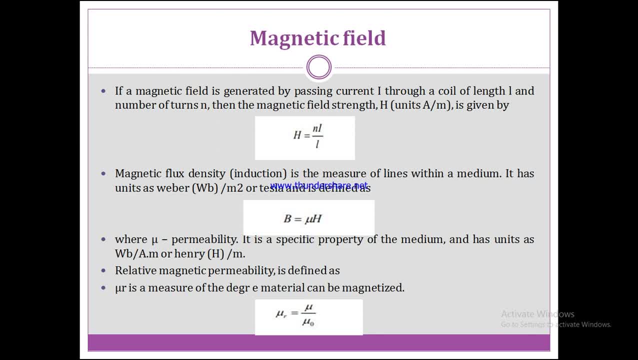 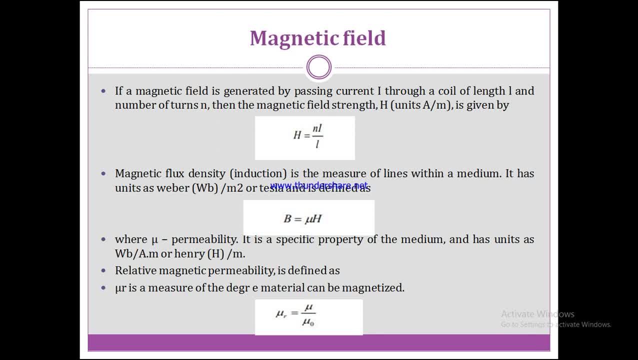 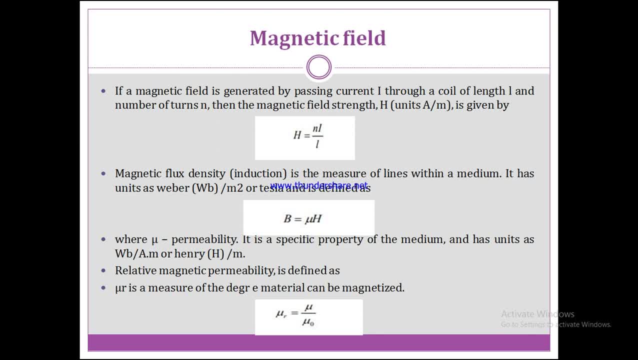 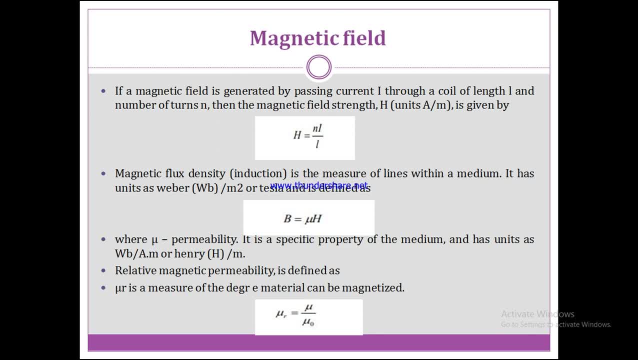 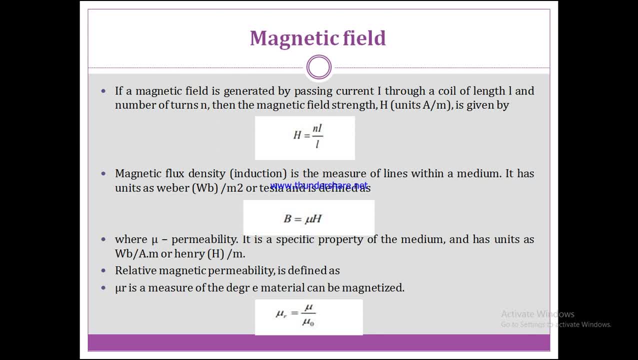 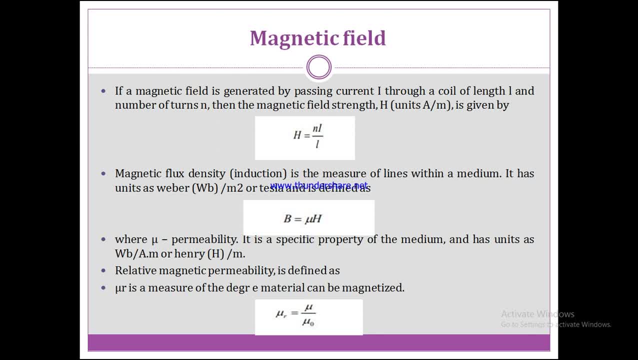 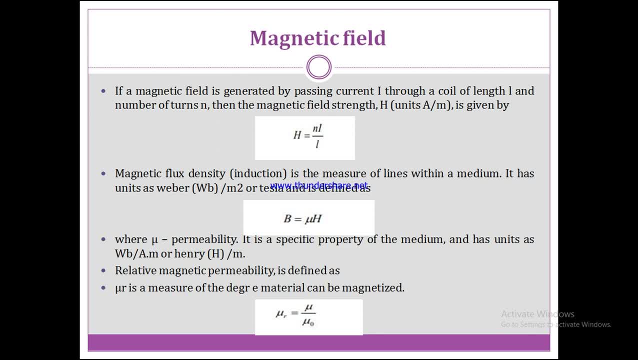 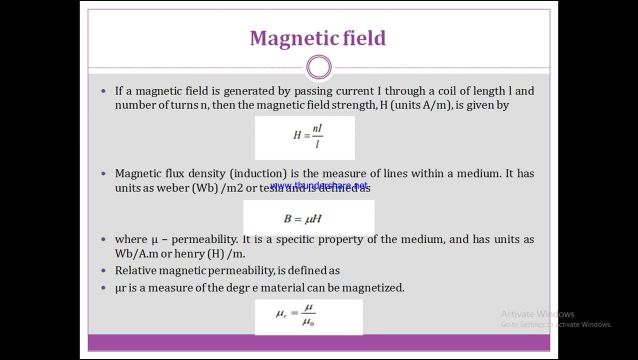 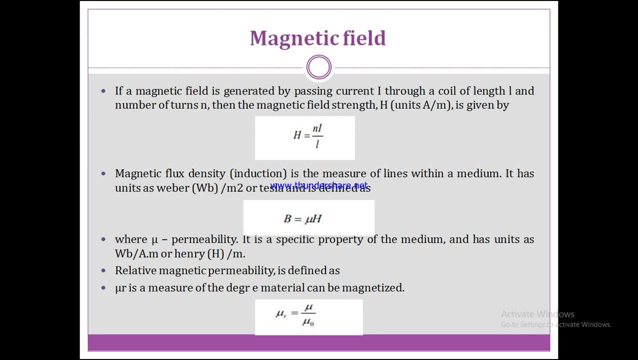 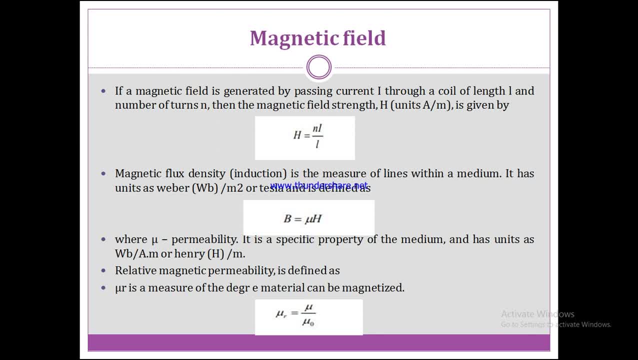 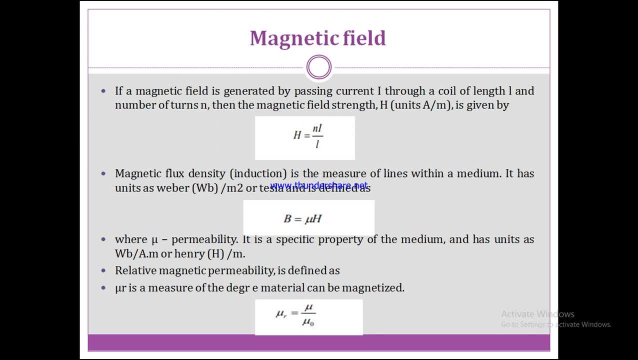 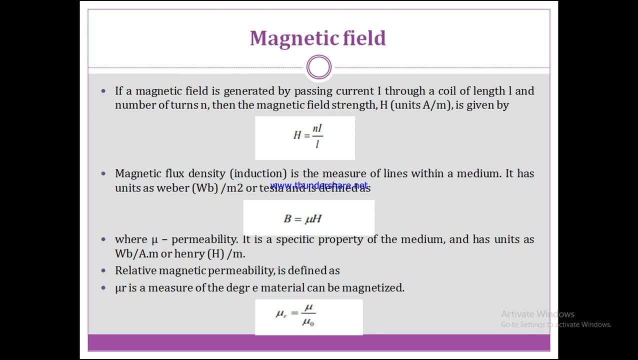 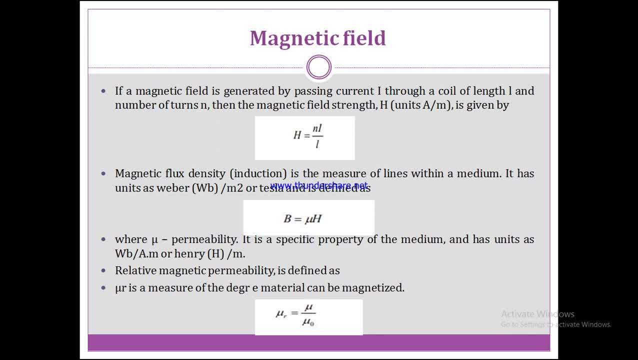 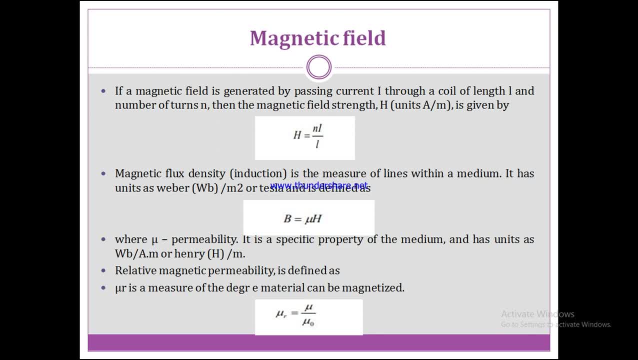 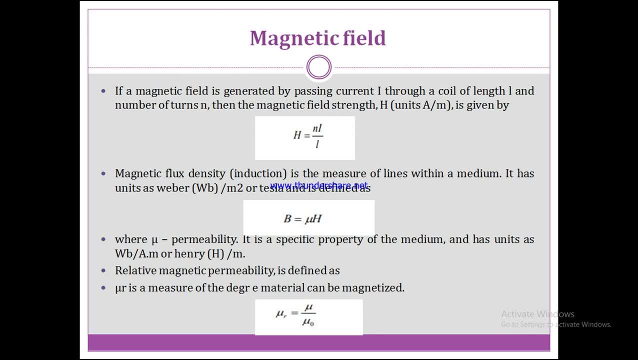 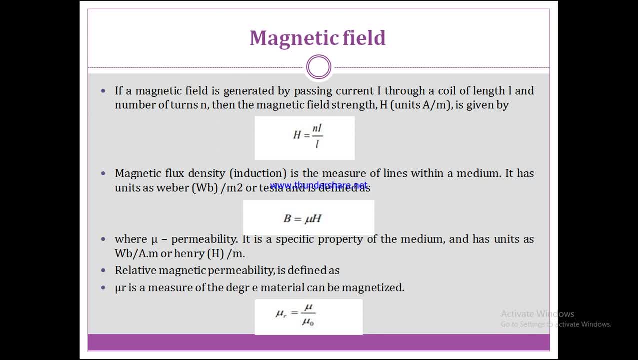 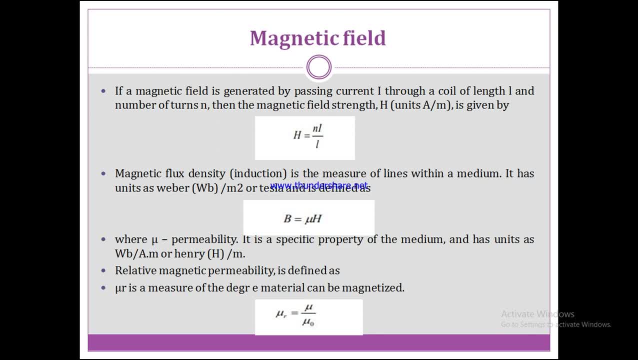 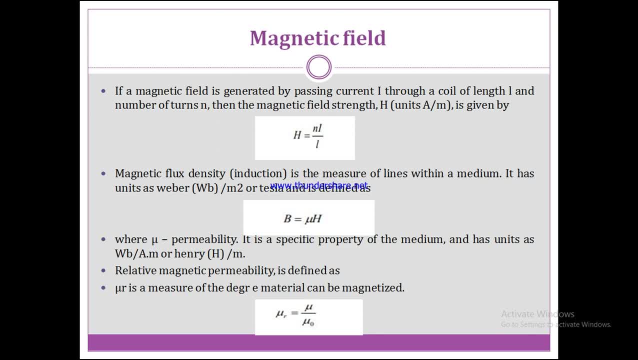 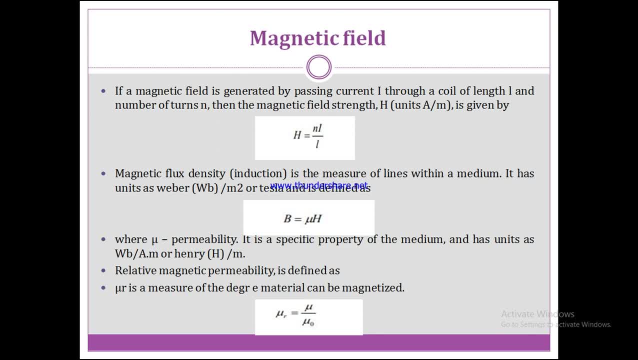 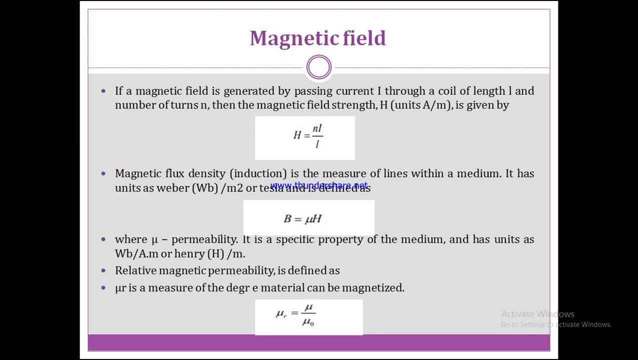 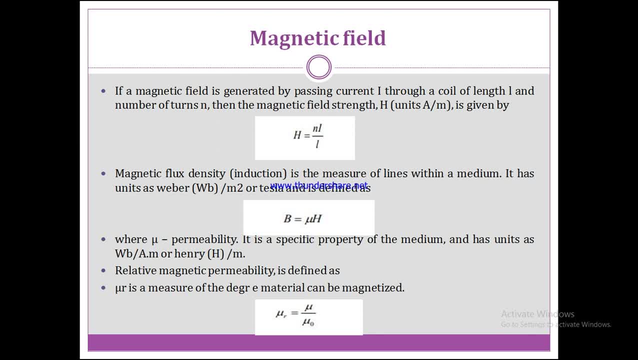 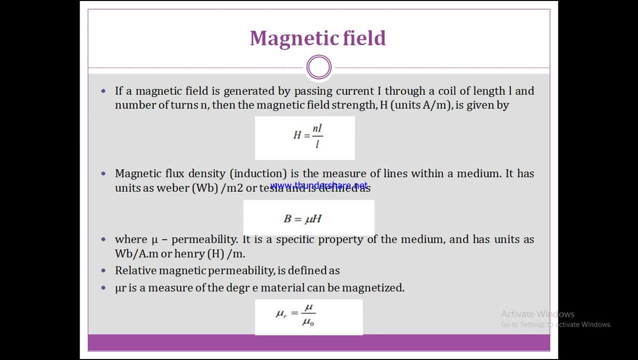 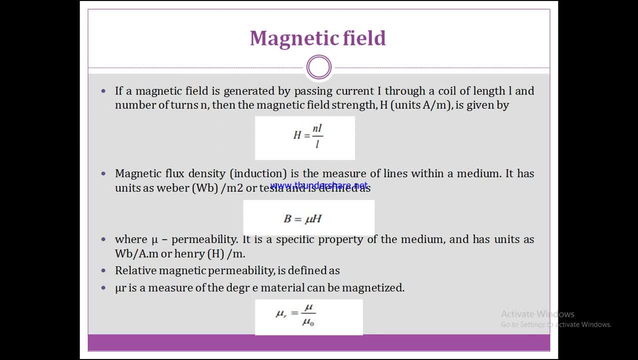 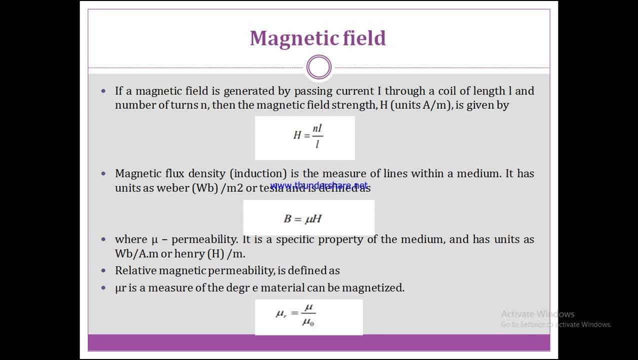 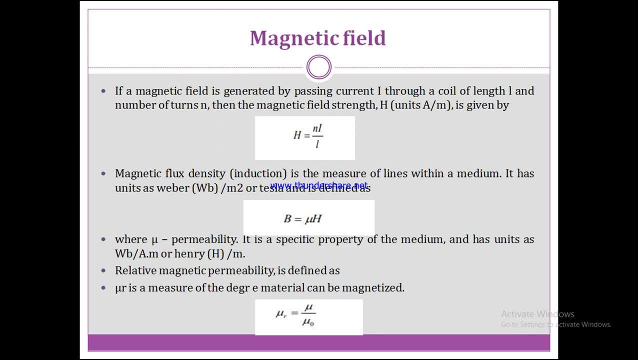 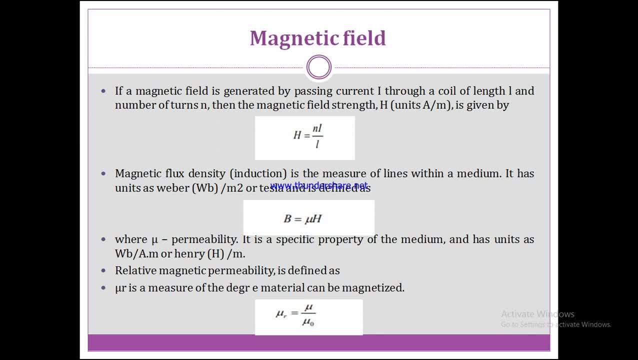 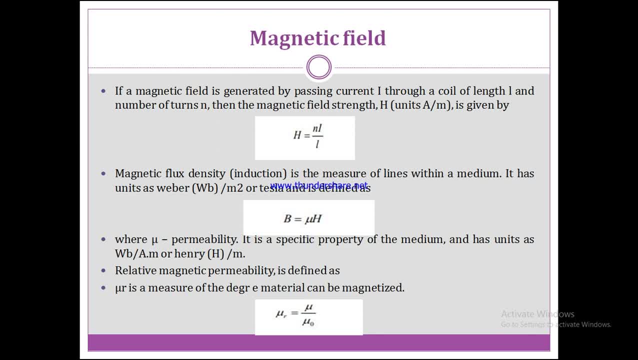 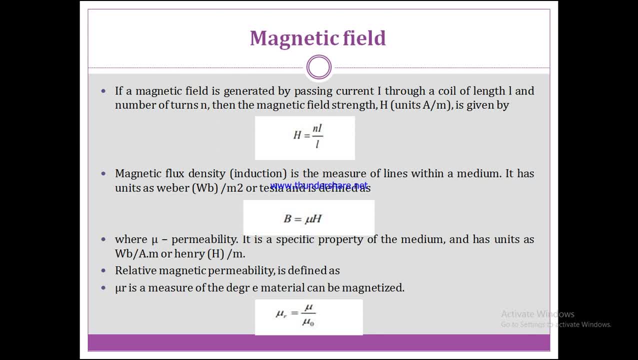 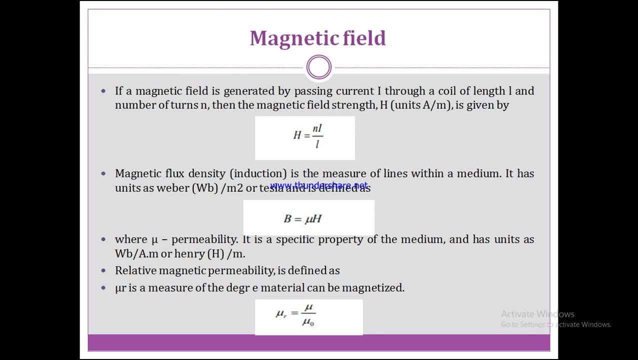 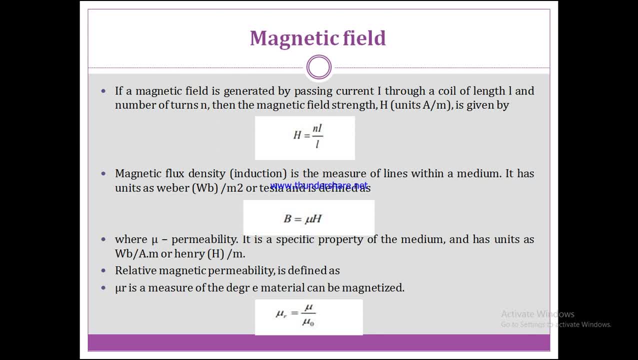 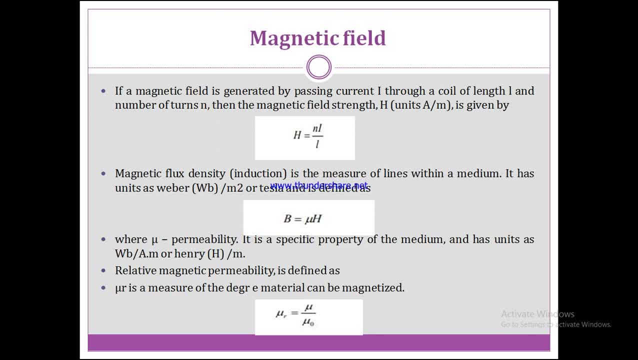 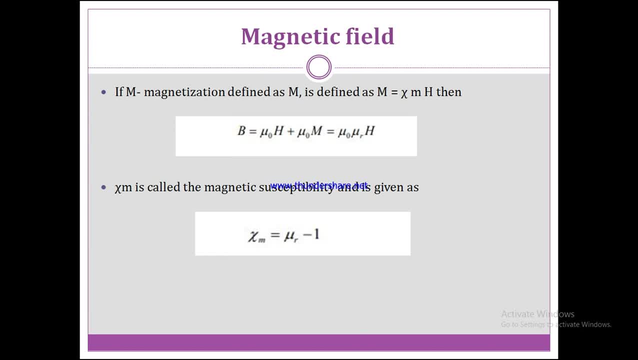 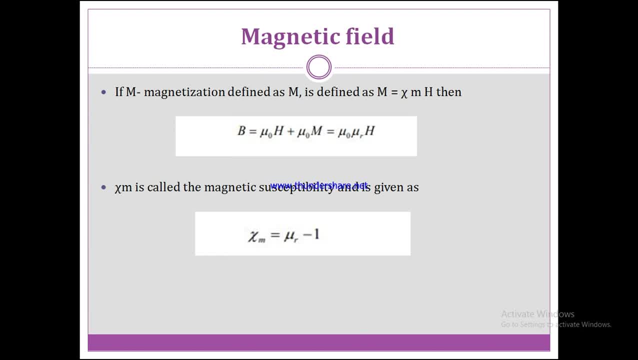 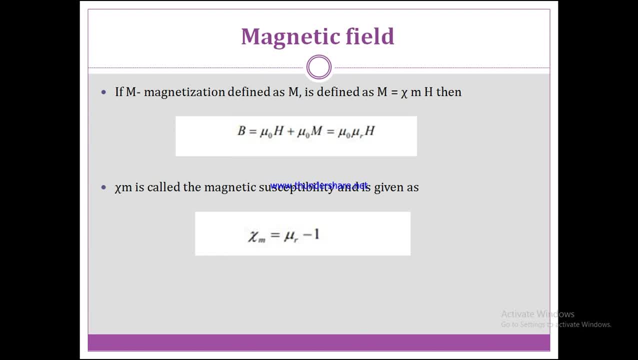 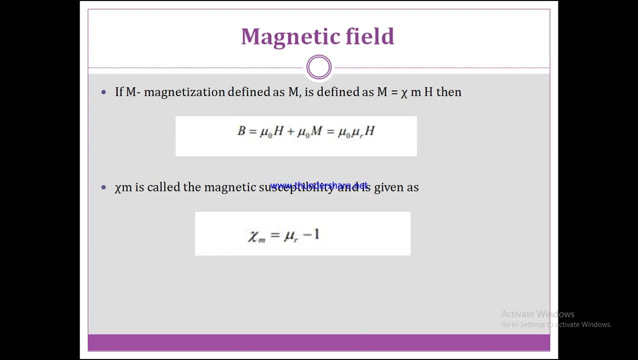 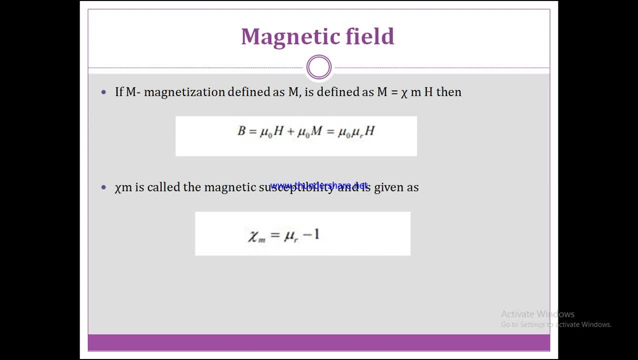 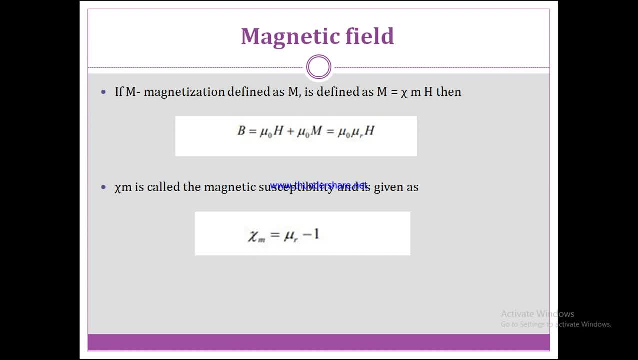 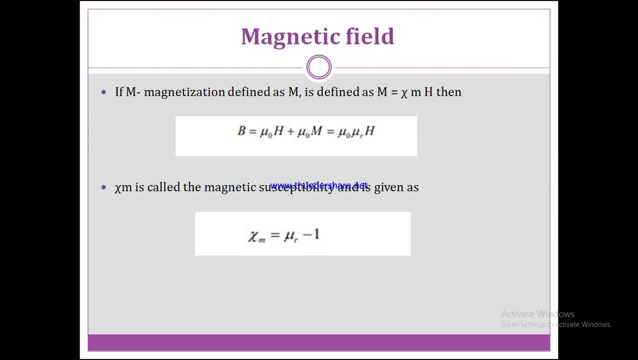 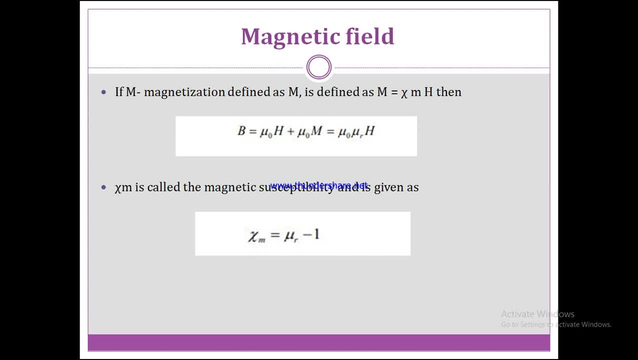 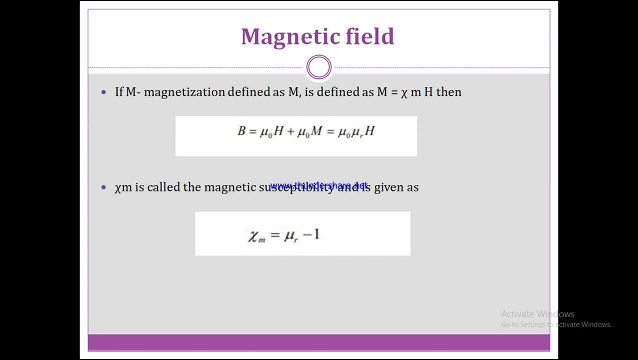 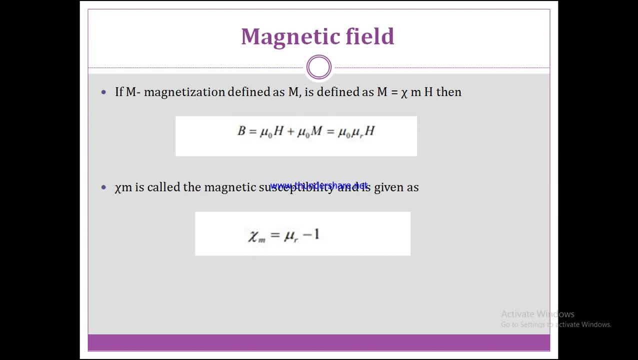 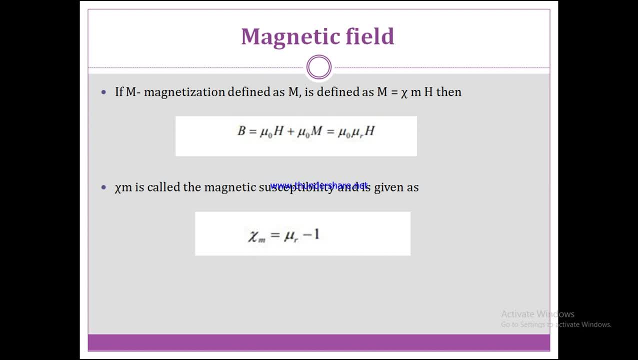 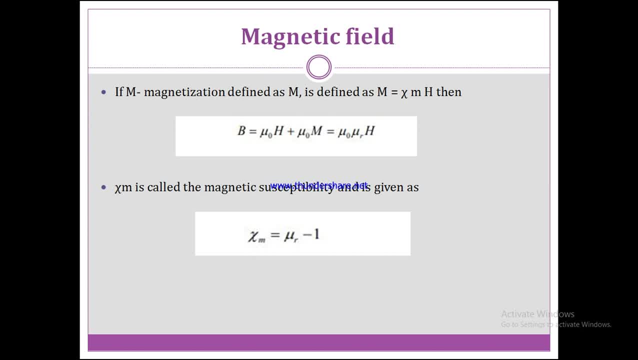 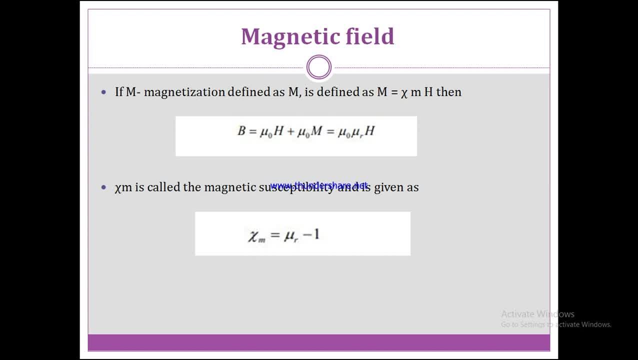 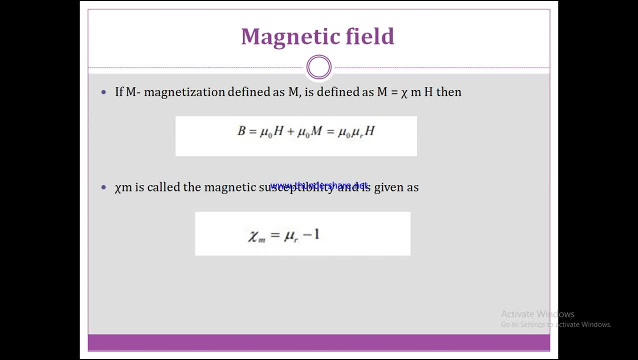 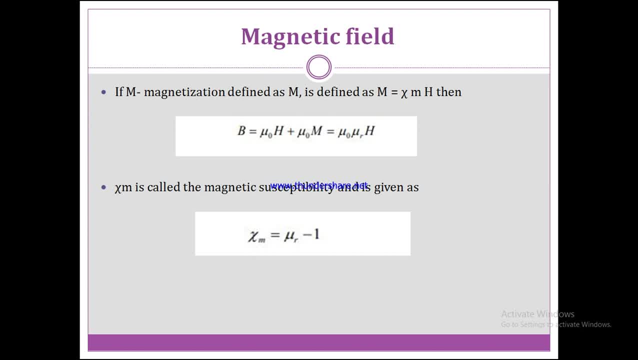 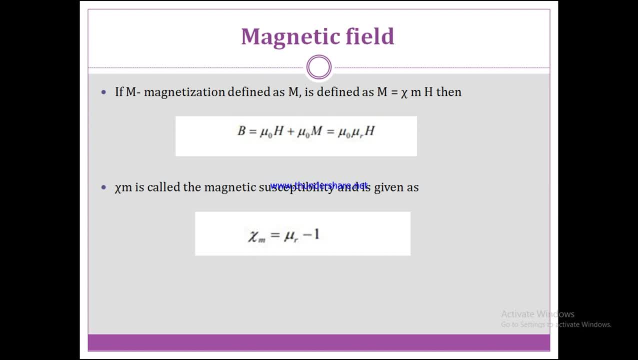 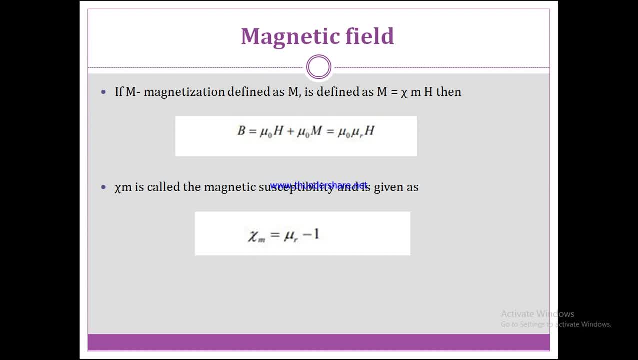 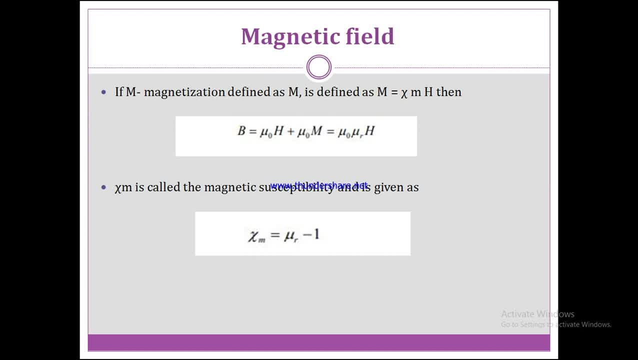